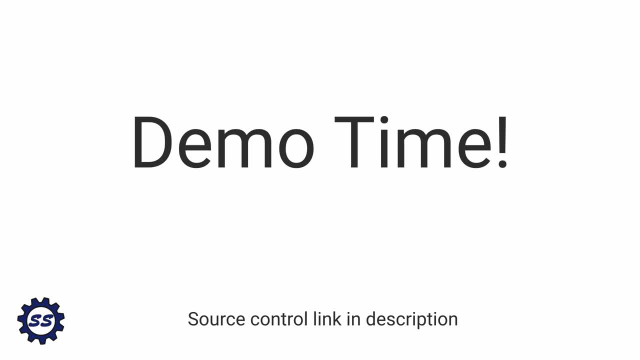 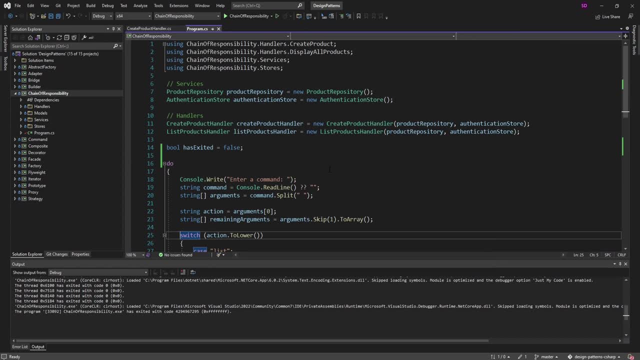 chain of responsibility pattern in our demo so that we can clearly see the benefits of it. So in this demo we just have a console application where we manage a list of products. So I feel like the best way to demo this is just placing breakpoints and we'll run through it. So here we go. So what? 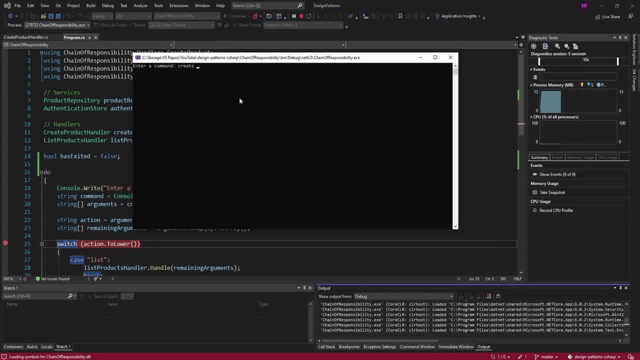 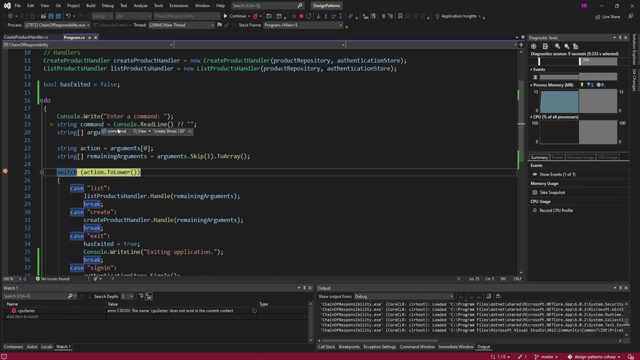 I want to do is create a product. So I'll say create, and the description of the product- These will be shoes and the price will say 120.. So here we go, We got our command that we typed in: create shoes, 120. Then we split that by the spaces and we have these arguments: So create, and then the. 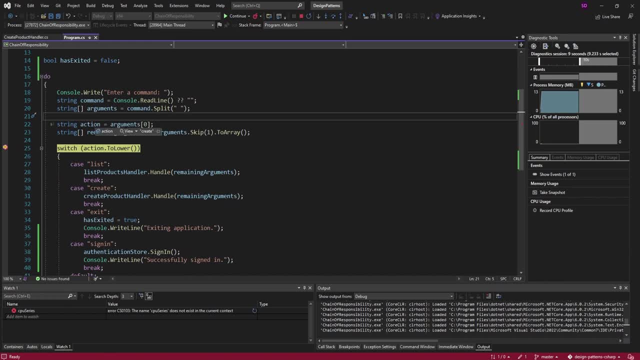 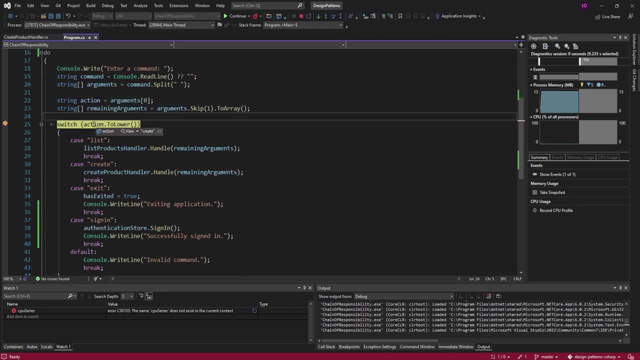 second item is shoes and the third item is 120.. The first argument is the action. So we want to create a product, and then we just have the remaining arguments for everything but the first argument, which was the action, and we use these later. So we go through this switch with. 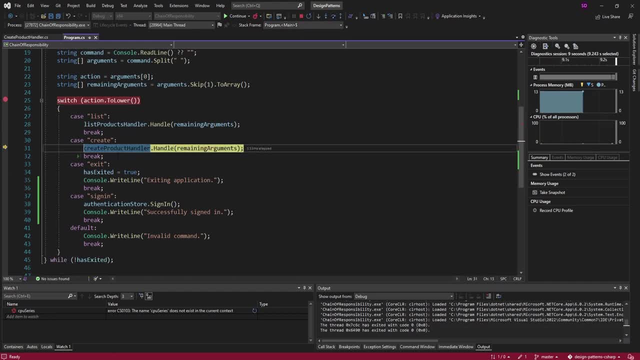 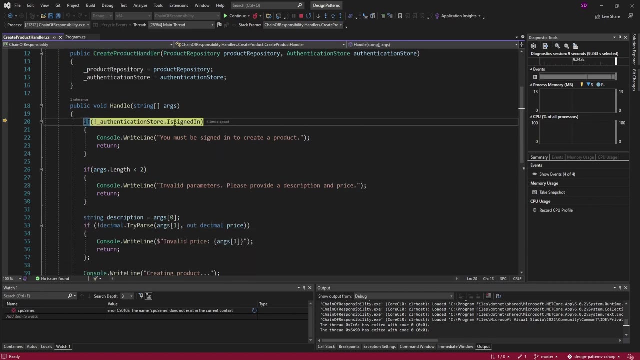 the action of create. So that causes us to enter this create product handler and we pass in the remaining arguments with the details of the product we want to create. So shoes 120.. So let's enter this. So we're now in this create product handler and the first thing we do is check if we're signed. 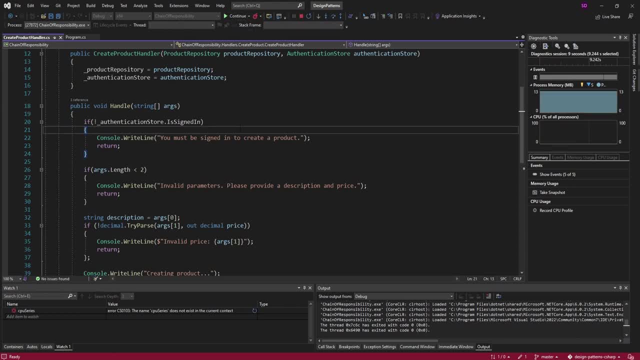 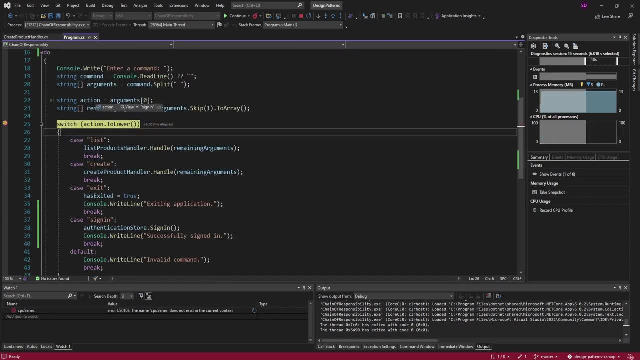 in. So we're in the create product handler and we're in the create product handler and we're in. So in this case we're not. So we say you must be signed in to create a product, So let's sign in. Another command. We'll say sign in. So, as we see, our action is sign in and then we enter the. 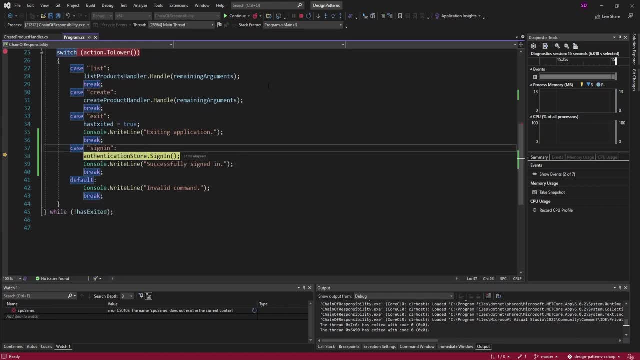 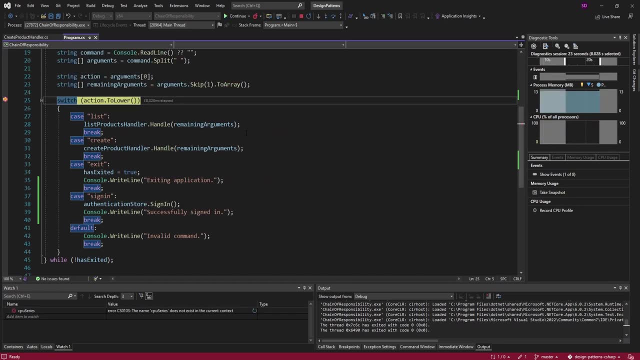 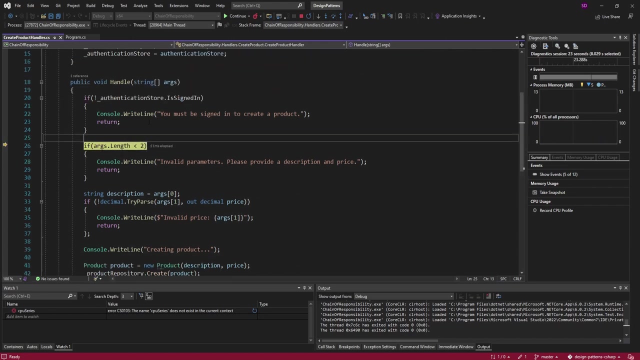 switch statement where we sign in through this authentication story. So let's do that, Successfully signed in. Let's try creating these shoes again. So run through that, We should get into our create product handler. This time we are signed in and we do some validation. 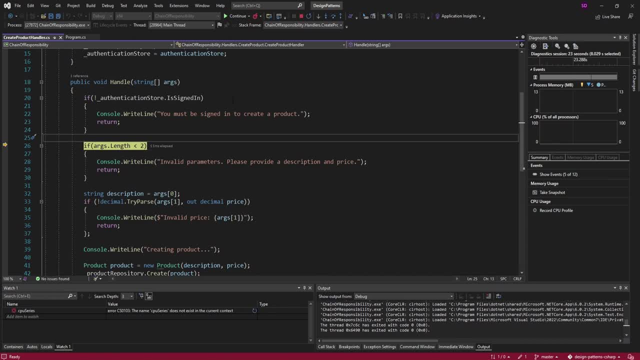 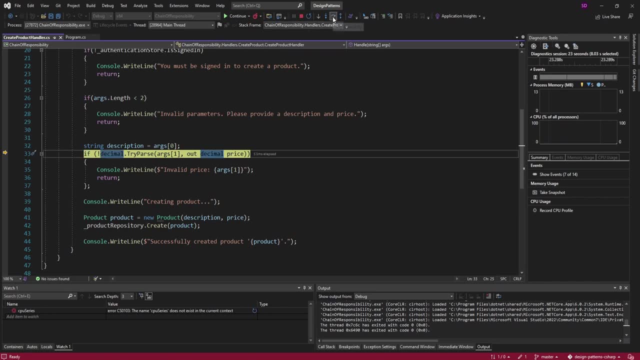 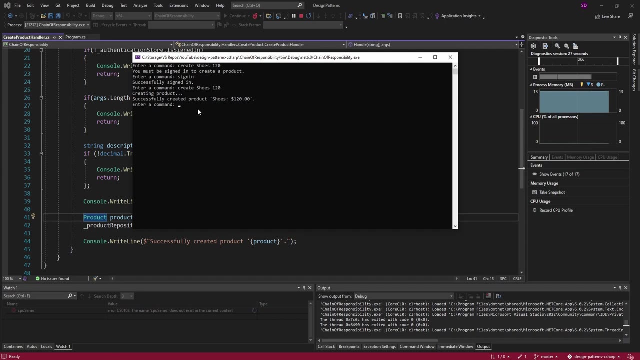 on these arguments. So we make sure we have the description and price, which we do. So we extract those, We validate the price is a number And then, since it is, we create the product and we successfully create it. So there we go: Create a shoes for 120.. So now, if I want to list all my 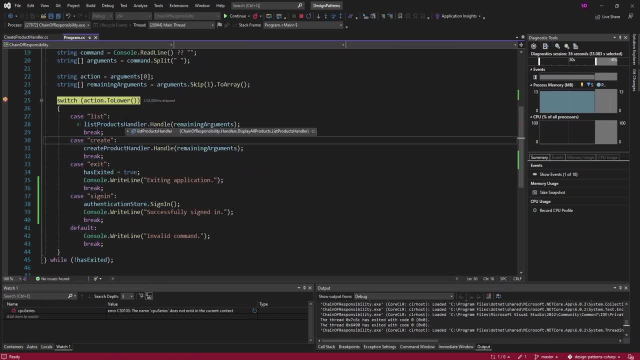 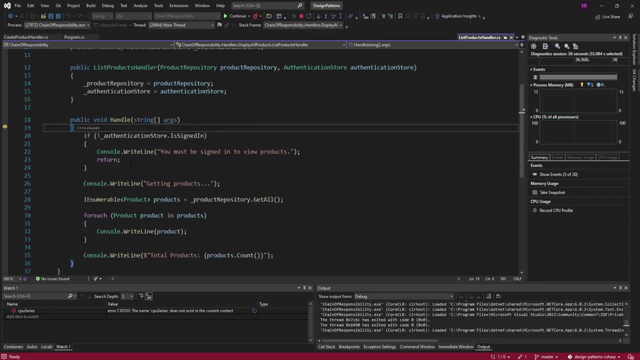 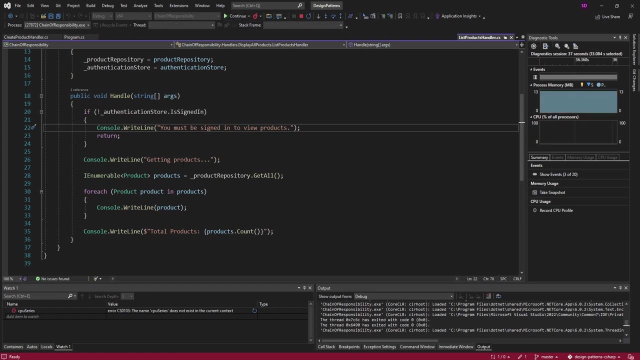 products- I can just say list- and we enter this switch statement again. Our action is list. So we get into this list product Handler, And here we go. We do the authentication check again, So you have to be signed in to view products, which we are. So we'll just write out all the products to the console And here we go, We. 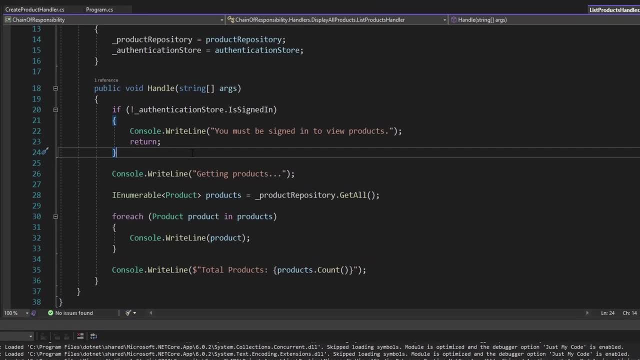 got our shoes for 120.. So at this point we are not using the chain of responsibility pattern And we have a few issues here. So for one, this create product handler and this list products handler. They both have to implement this authentication logic, So we have some duplication. 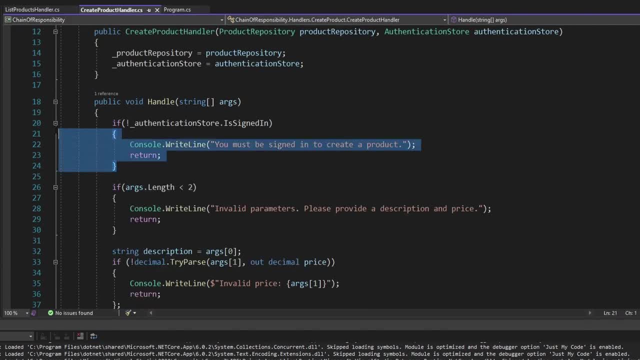 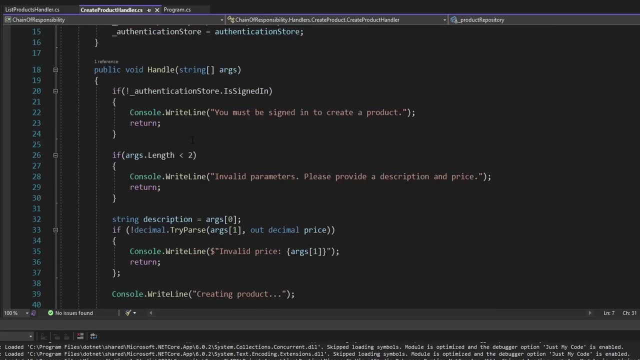 here, And also both of these products have to be authenticated, So we have to implement this. Mrs Handler's have force themselves to be concerned with authentication, whereas in reality you would think the create product handler would just be concerned with creating a product. So in my opinion, this create product handler is doing too much by handling authentication. 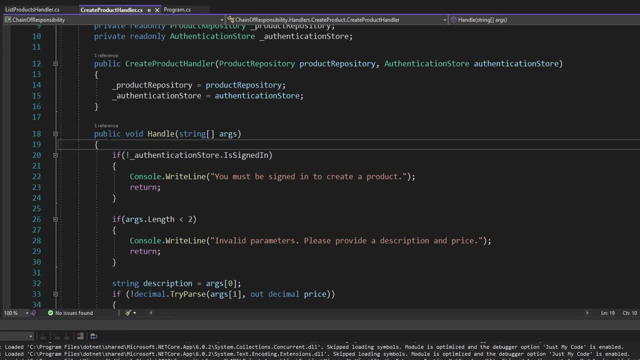 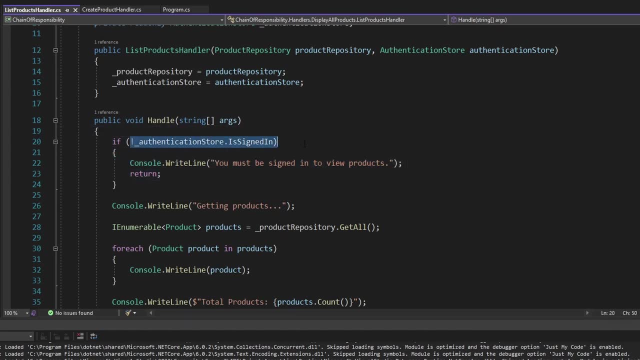 And who knows, maybe we would want to disable authentication to create a product or, more realistically, to list products. If we wanted to disable authentication, then we'd have to come into this list products handler and delete it. So this solution isn't very flexible and we have some code duplication between our 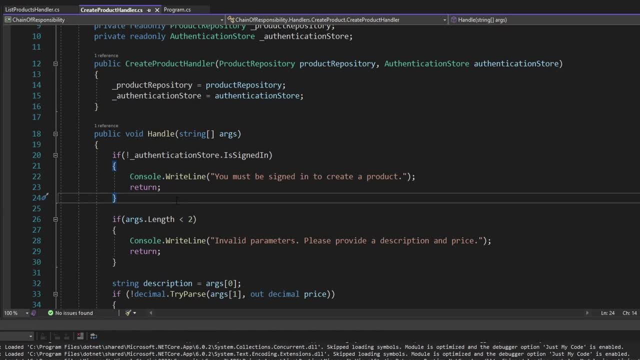 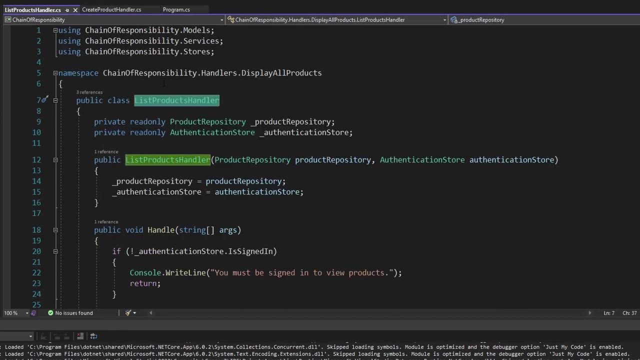 handlers. So ideally, I would want to leverage the chain of responsibility pattern by having a chain of handlers where the first handler would handle the authentication and if we're authenticated then we'll move into the next handler, which might be for creating a product or listing products. So 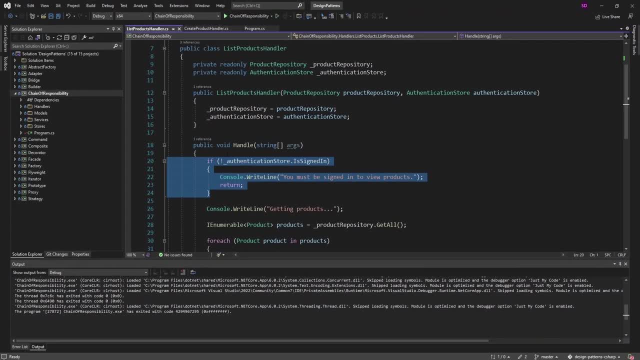 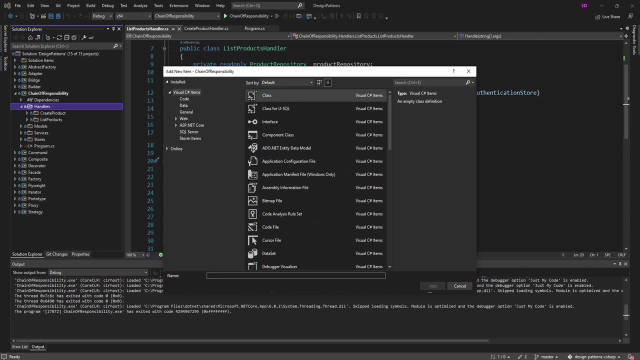 that being said, let's create our authentication handler, which will handle this authentication logic. So in our handlers folder we'll just throw another handler in here, We'll call this the authentication handler and we'll have a handle method on here. So it'll just be a void handle. 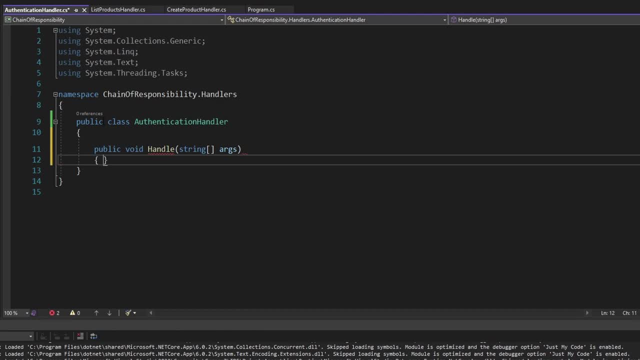 method and it'll take in args. So same kind of interface that these other handlers have. and then in this handle method of the authentication handler, we'll handle. the is signed in check. So let's copy all this into the authentication handler. So if we're not signed in, we'll write it out to the console. We'll make this more generic. We'll 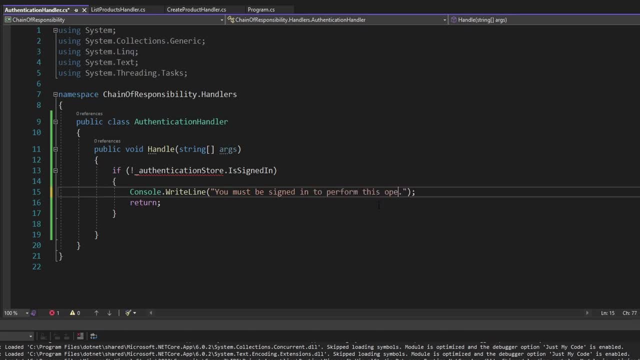 just say you must be signed in to perform this operation. But then if we are signed in, then we want to forward the request to the next handler in the chain. So we're going to need that next handler. So it'll be something like next handler which will handle the request and we'll just pass. 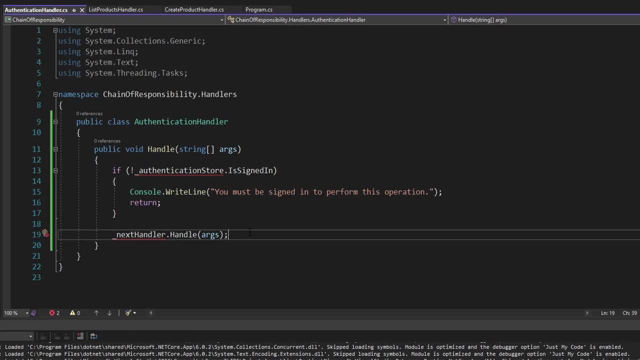 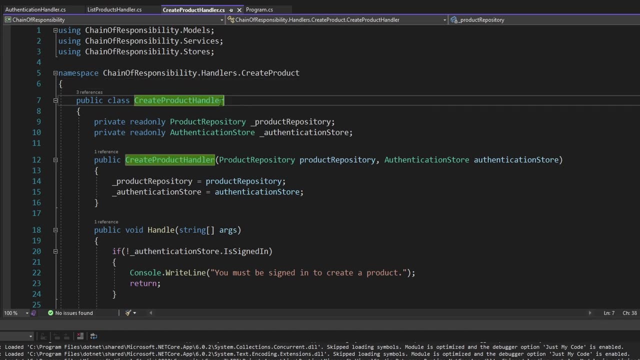 in all of those args. So this next handler is going to be, in our case, either the list products handler or the create product handler. So we're going to have to depend on something more abstract if we want to support both of these handlers. We can't just depend on these concrete types. So in that, 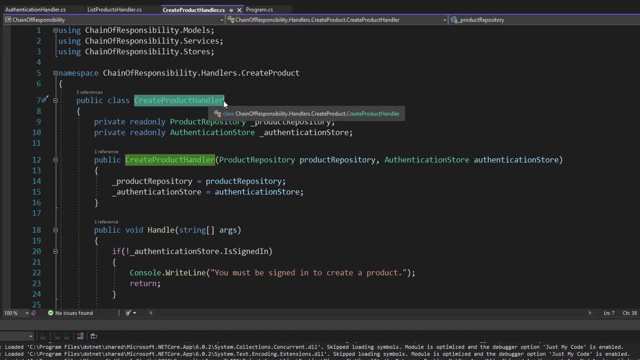 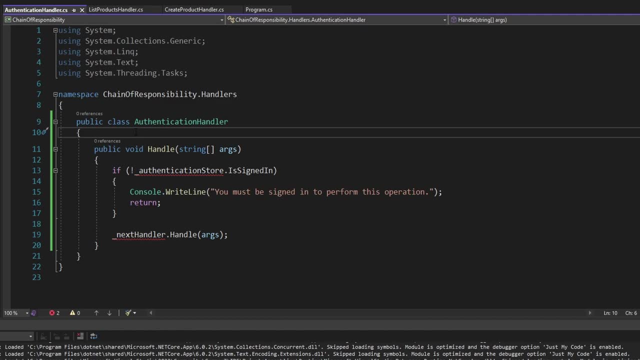 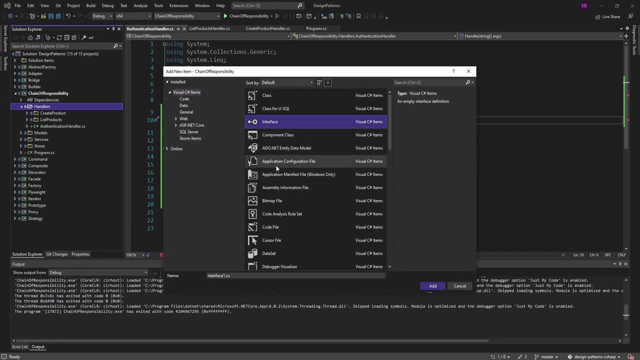 case, we're going to create some kind of I handler interface that both of our handlers can implement and then our authentication handler can reference that interface and support really any handler that implements the I handler interface. So let's create that interface called the I handler. 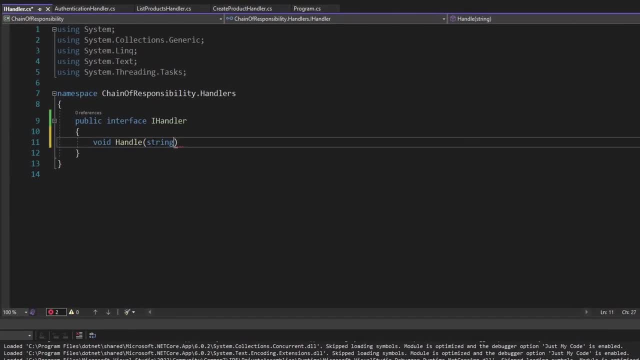 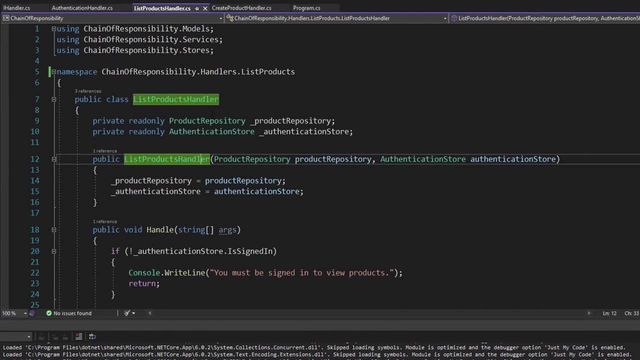 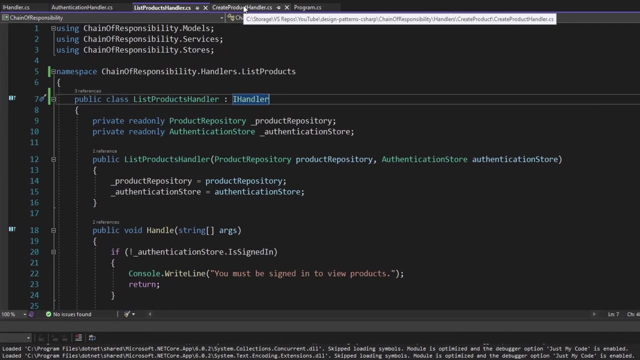 And it's just going to have a void handle method that takes in an array of arguments. So same function signature that our handlers already implement. So let's implement the I handler interface on both of these handlers. So list products handler implements it already as well. 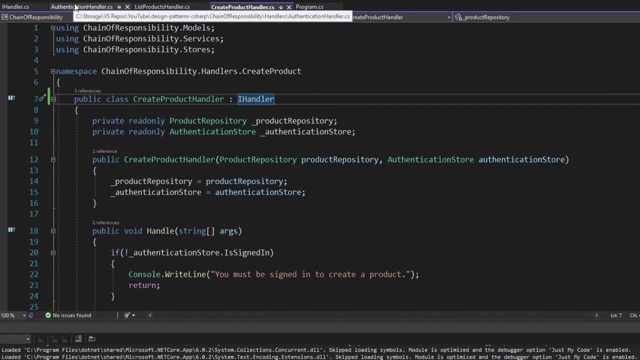 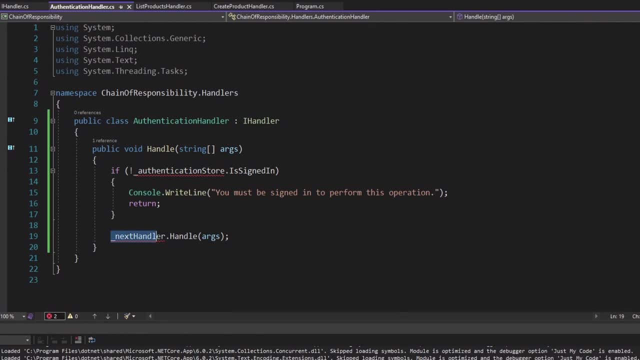 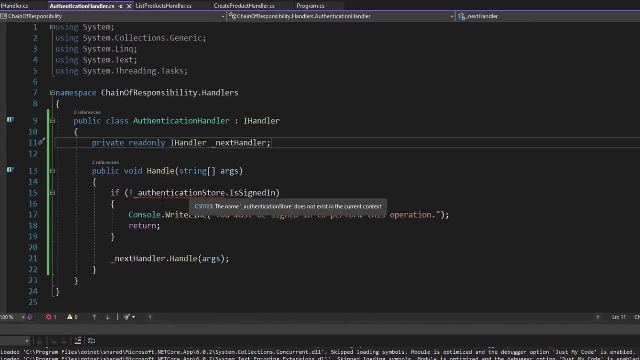 as the create product handler. And while we're at it, the authentication handler can also implement it. So now that we have this interface, that interface is what we'll depend on for this next handler field. So we'll have a field for the next handler. It'll be an I handler, And then we also need the authentication store in here. 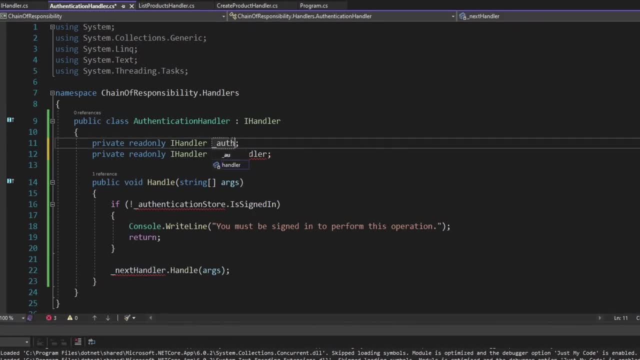 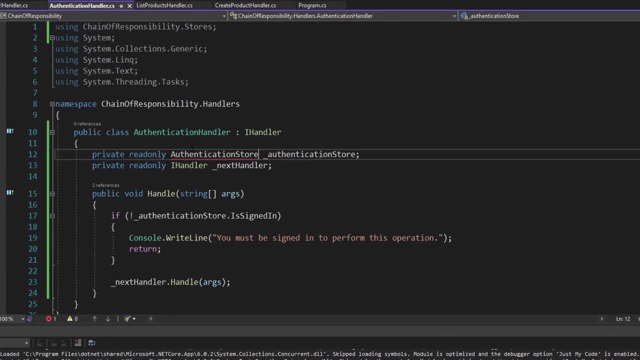 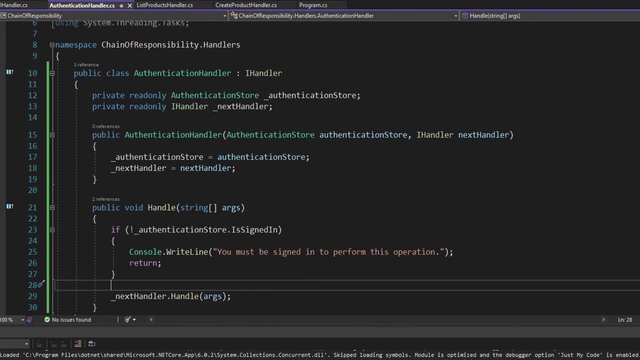 so we can check if we're signed in or not. So let's get that as a field as well. The authentication store: Let's import that, And we'll get both of these passed through the constructor. So now this should be everything that the authentication handler needs to do. Now we just need to use it. 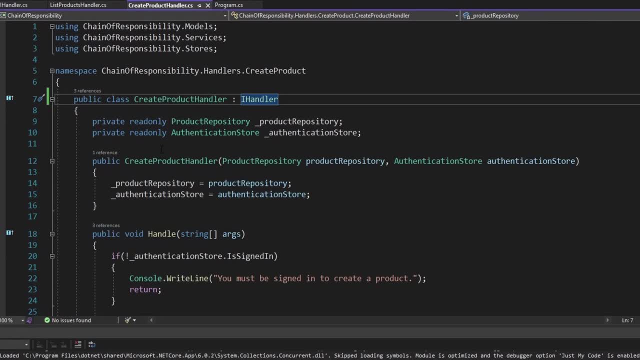 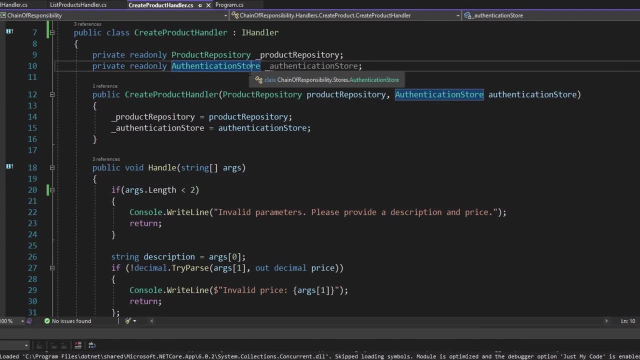 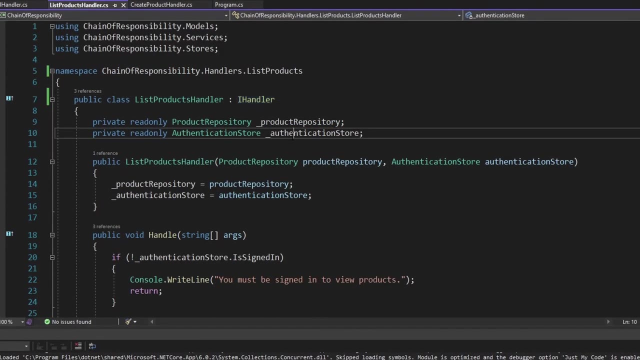 So let's move into our other handlers and remove the authentication checks here. So now the authentication check is going to be handled higher up in the chain. So in that case we don't even need the authentication store passed in to these handlers anymore. And same goes for the list. 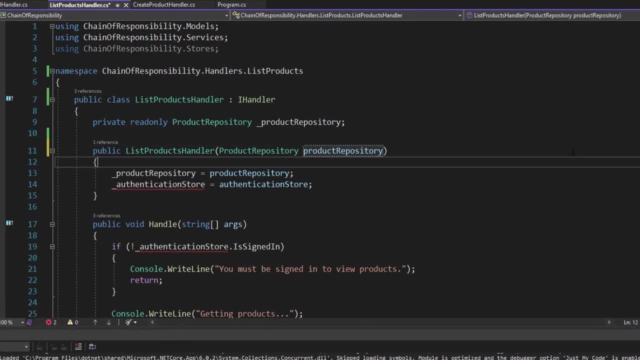 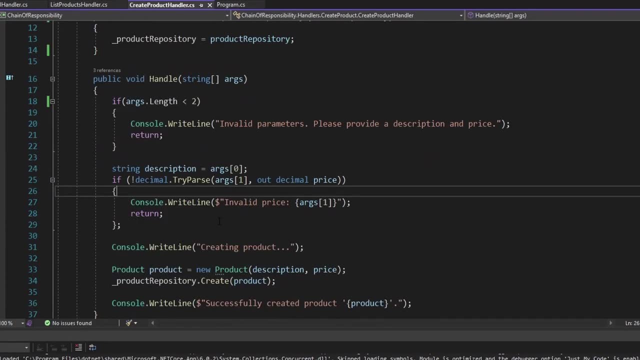 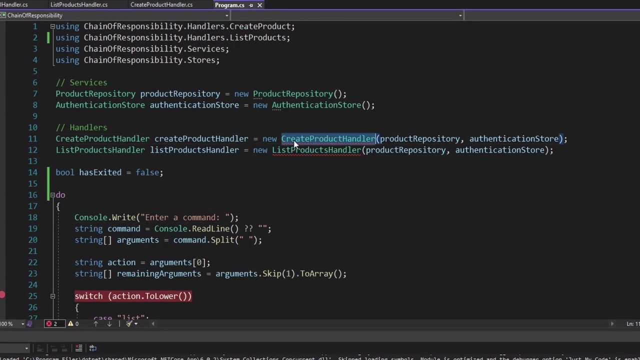 products handler. Let's remove the authentication store and remove the authentication check. So now these handlers are a bit thinner and now we can simply enable it again force authentication higher up in the chain. So here in our programcs we instantiate our create product handler and our list products handler. But before we execute either of these, 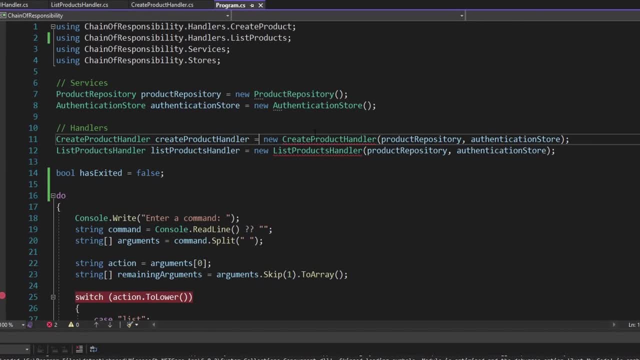 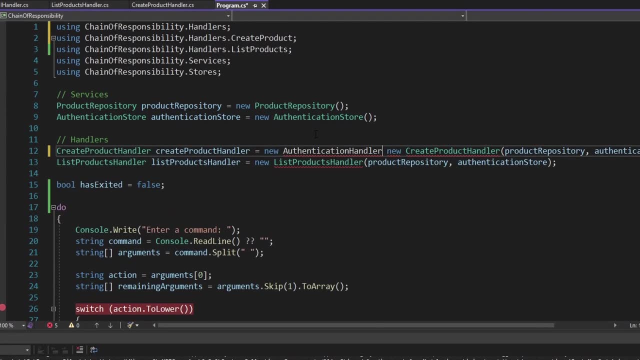 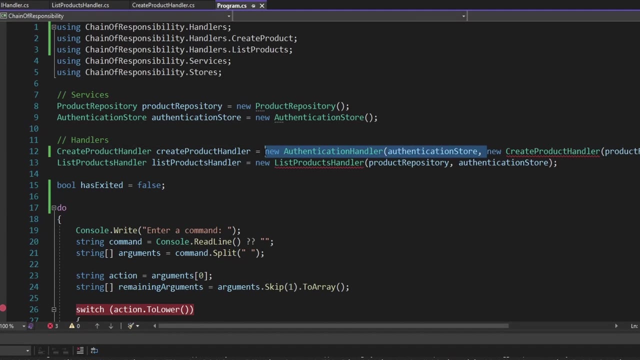 handlers. we want to check authentication first. So we're going to wrap these handlers in the authentication handler. So let's import that and pass in our handler. We also need to pass in the authentication store. and same thing for the list products handler We want to wrap. 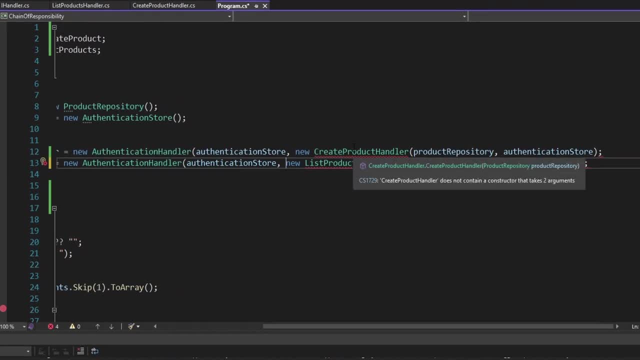 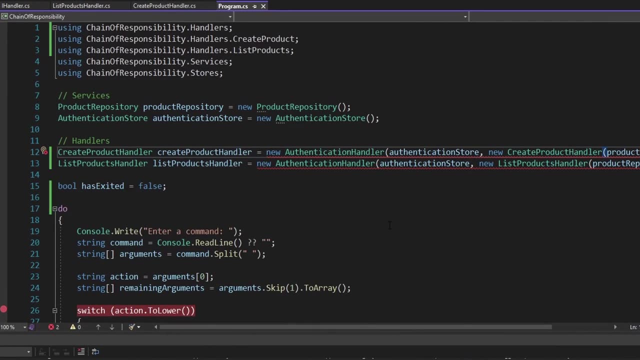 that with the authentication handler and then let's clean up these constructors So we no longer need the authentication store pass to either of these handlers. So should be good on instantiating these handlers. The last issue we have is that this create product handler isn't a create product. 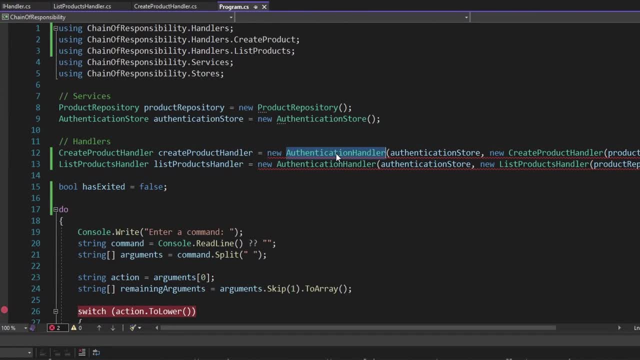 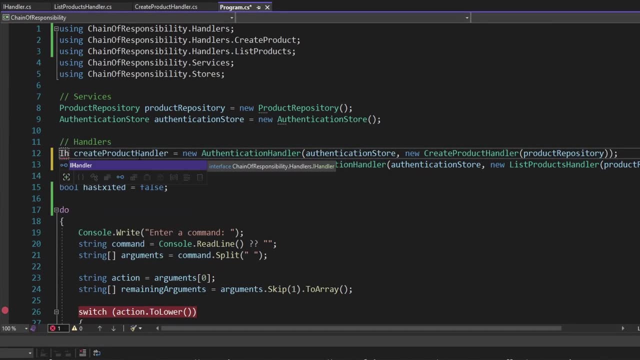 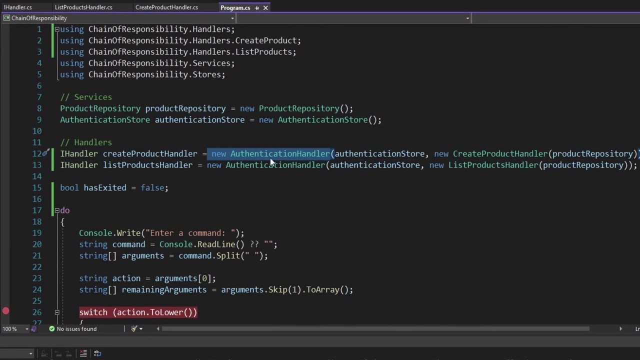 handler anymore. Now it's an authentication handler. but we don't want to just make these authentication handlers So to make it more flexible. we just want to depend on the I handler interface. So now it doesn't matter if this outer handler is a create product handler or an authentication handler or any handler that. 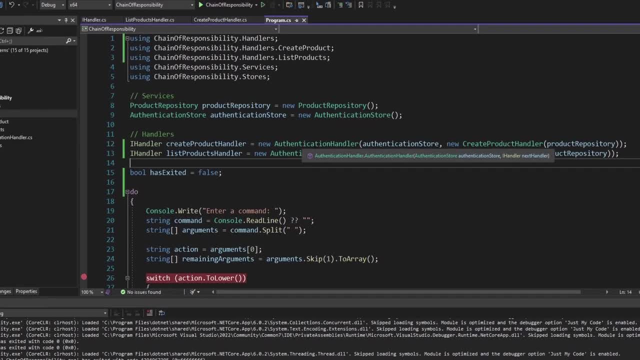 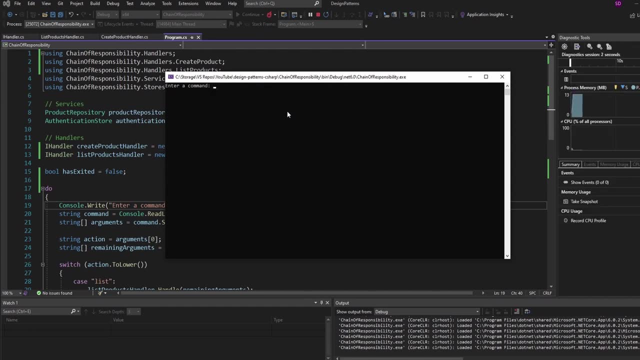 we create in the future. All it needs to do is implement the I handler interface, which this already does. So at this point we should still have authentication enforced, even though our specific handlers aren't enforcing it on their own. We enforce it higher up in the chain. 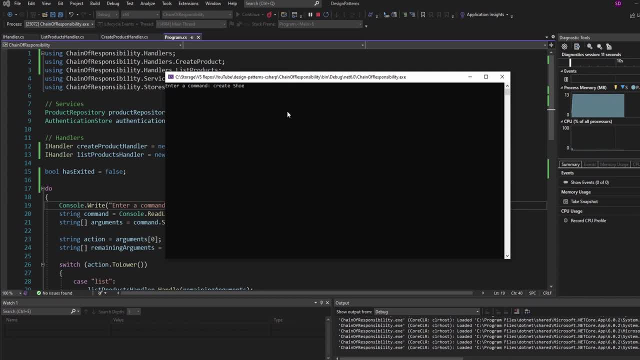 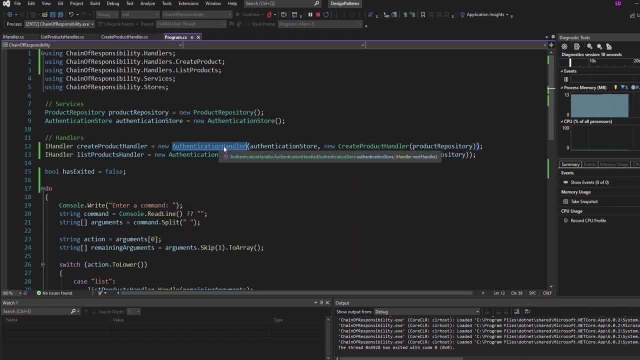 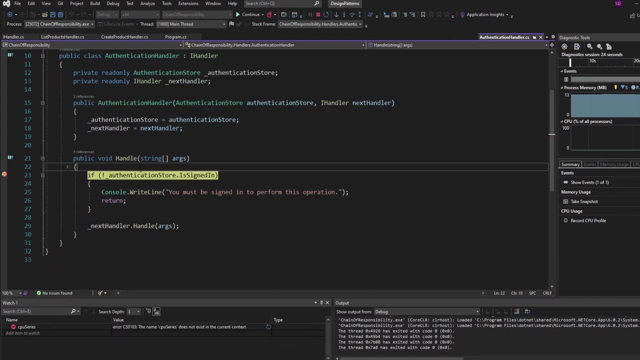 So let's try creating a product: shoes for 120.. But of course we must be signed in to perform this operation. So this authentication handler seems to be working. Let's put a breakpoint down and try this again. So here we go, Hit the authentication handler, We are not signed in and we simply exit. 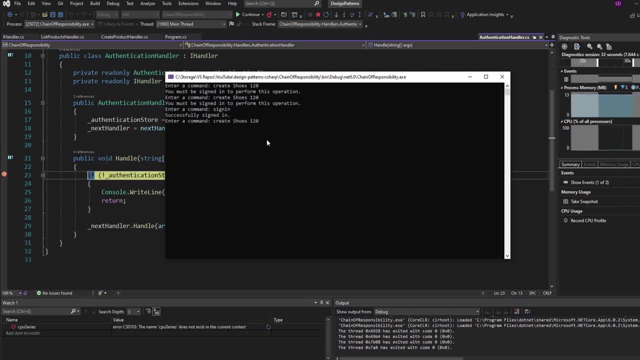 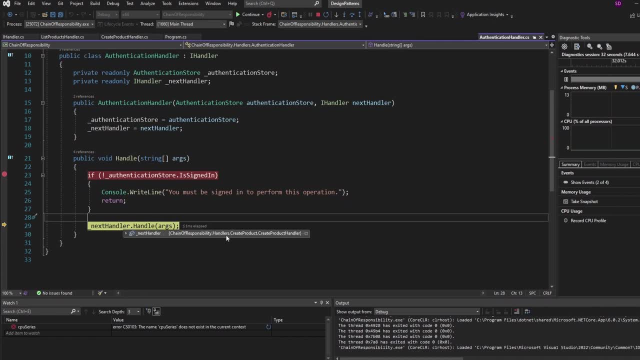 early. So let's sign in and try it again. This time we are authenticated, So we pass the request along to the next handler. So let's try this again. So we pass the request along to the next handler, Which in this case, is our create product handler, And we can create the product. There we go. 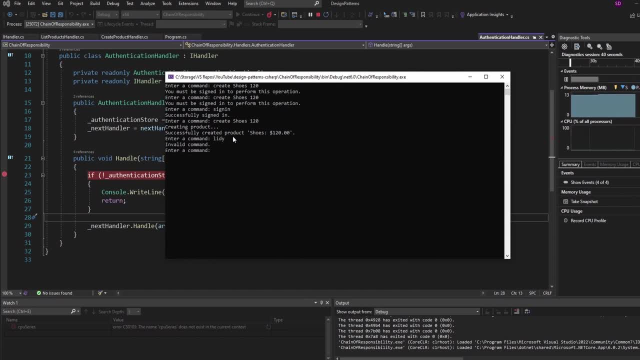 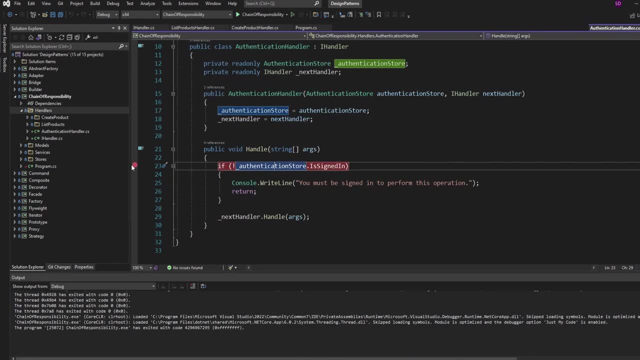 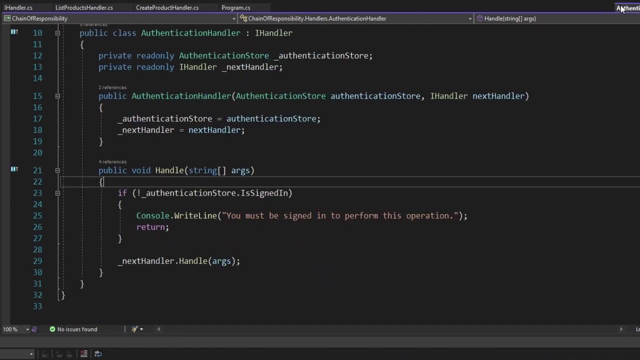 And let's try listing out the products. So list, Whoops List. We are signed in and we write out all the products. So this handles the first issue where we were duplicating the authentication logic between both of our handlers. So we now have this simple, reusable authentication handler. 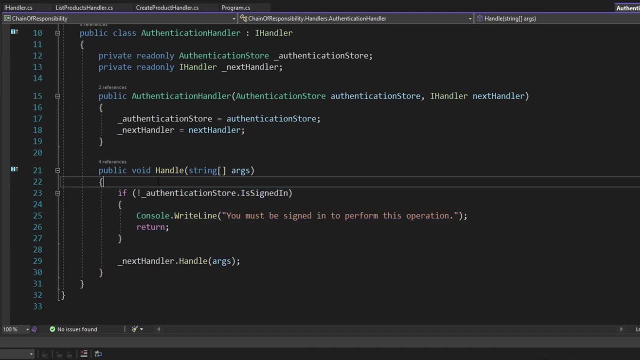 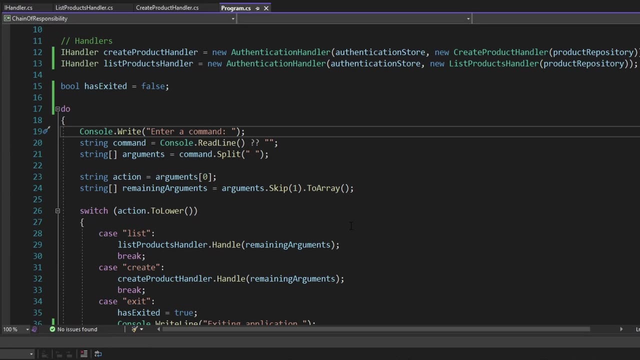 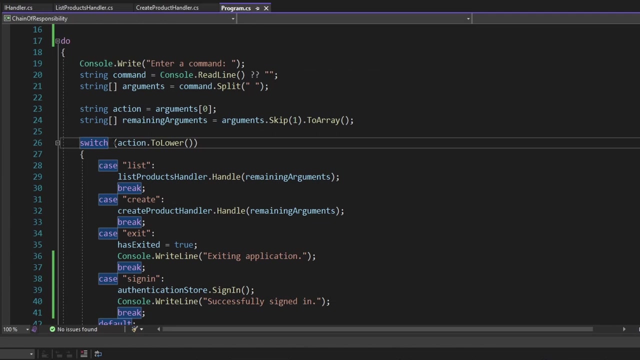 that focuses on one thing, which is just authenticating The user. So now that we've implemented this authentication handler and we're already starting to see the benefits of the chain of responsibility pattern, let's continue and see if we can enhance our chain of handlers. So here in the switch statement, where we read the action that we want, 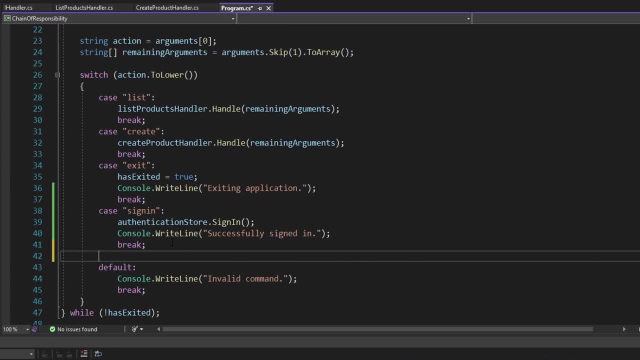 to perform. I want to add another action: to sign out. So we're going to have another case down here for sign out And for that we're just going to call sign out on the authentication store And we'll say successfully signed out. So we've made this change. It was quite simple. But what I didn't 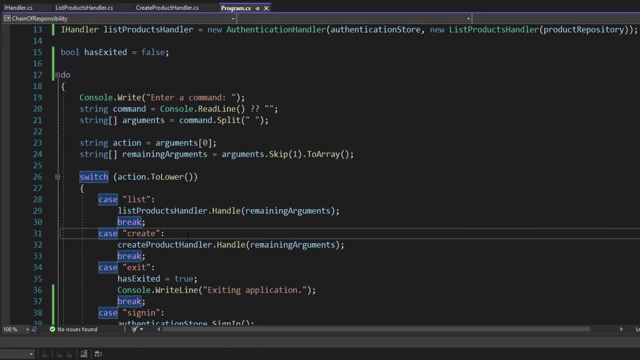 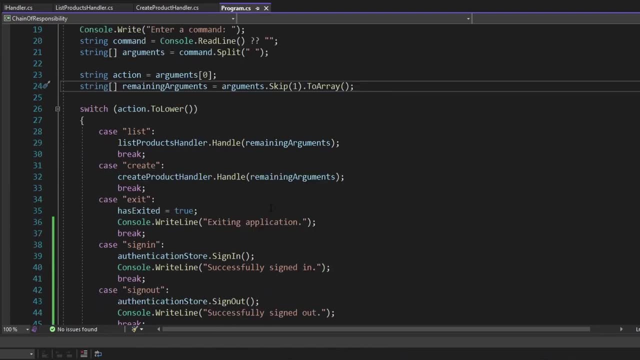 like about what we did is that we had to come into what I would consider the client part of the code, because this is where we really get into interfacing with the user. We had to come in here and directly add this and change this code. So, with that in mind, I feel like our client is. 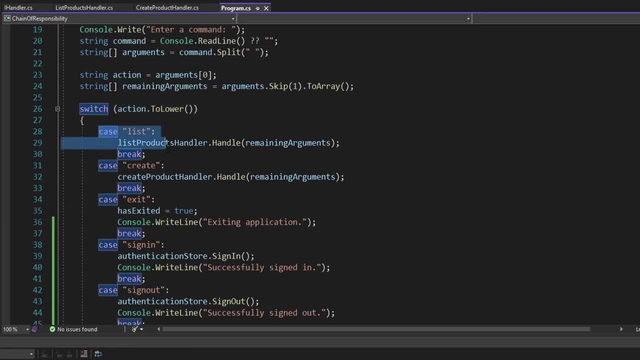 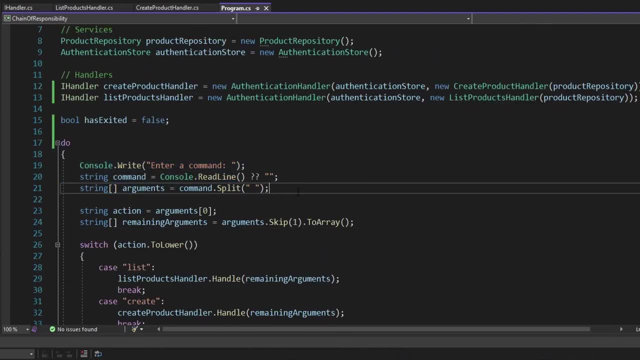 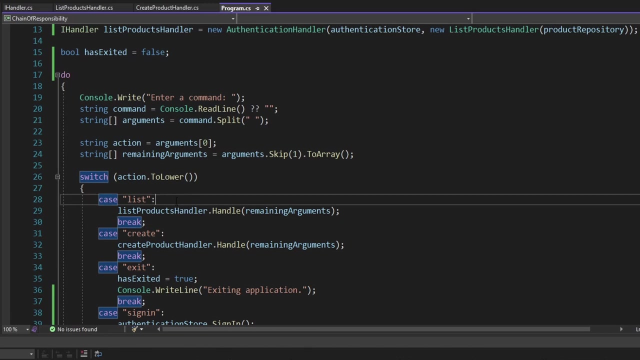 doing too much. It has to read the action and then determine which handler or which code to execute. So all the client should do is read the command that we type in and then pass it into our chain of handlers. It shouldn't be so concerned with determining which specific handler to pass into. 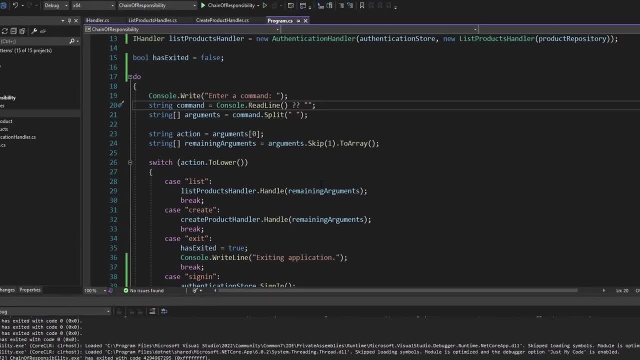 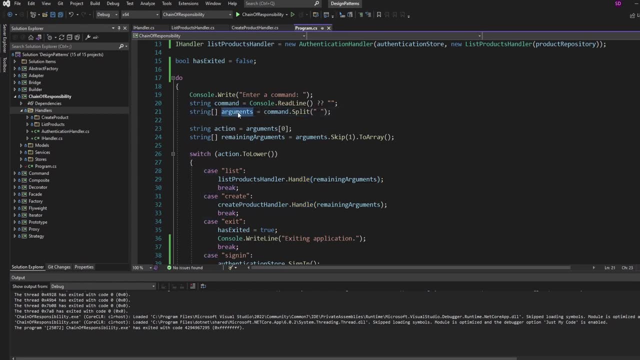 So, that being said, we're going to have a root handler that'll act as the entry point to our chain of handlers And all it's going to do is take in our array of initial arguments. So let's create that handler in our handlers folder. I guess we'll just call this the root. 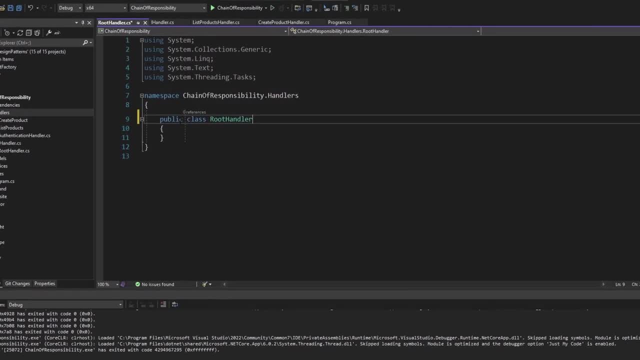 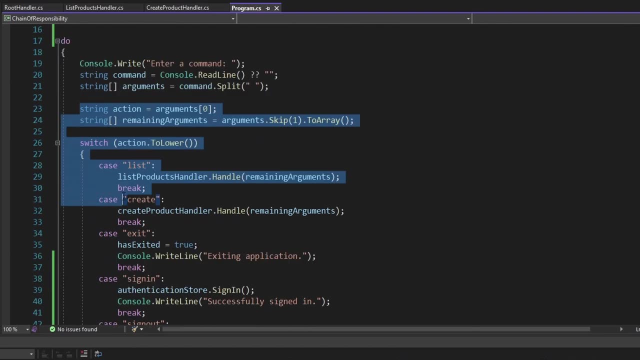 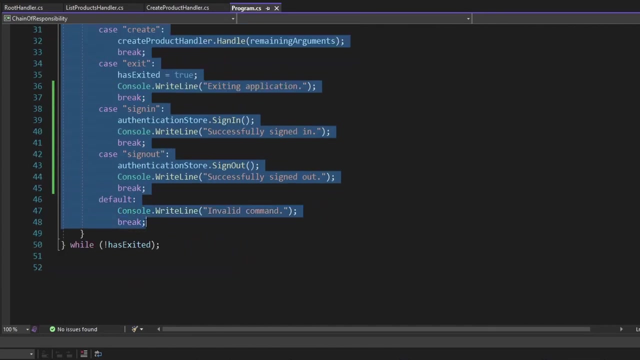 handler. That's a decent name. So let's create that, Let's implement our I handler interface and let's move into our programcs and move in as much as we can. So all I want the client to do is pass in these arguments to the handler. So we'll grab all of this. So where we extract the action and remaining 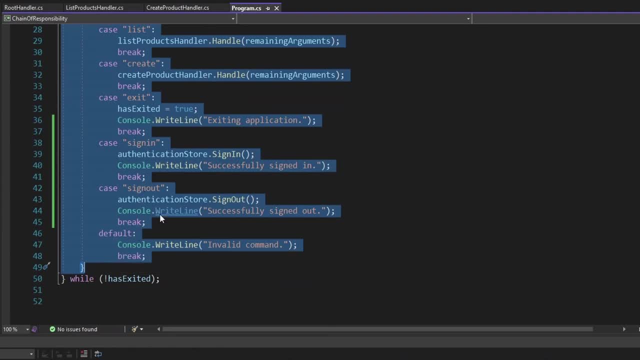 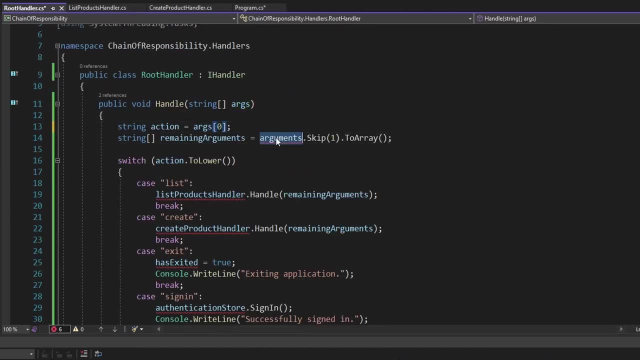 arguments and go through the switch statement. Let's cut that out and paste that into the root handler. So here we go And let's make sure we use our args parameter, And then we're going to need some handlers passed into this root handler. So first we're going to 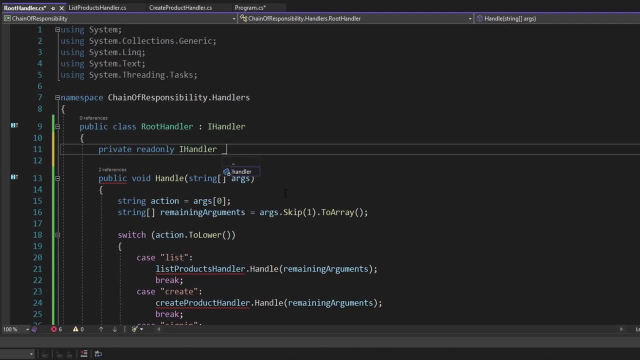 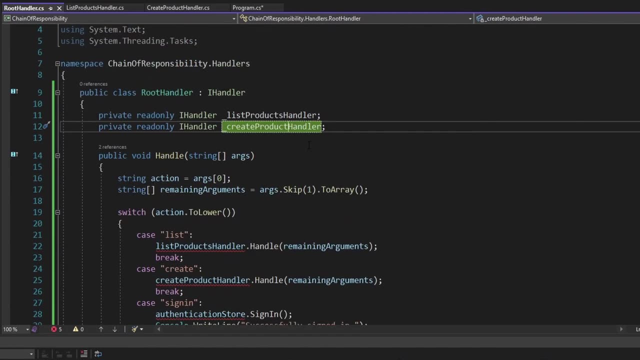 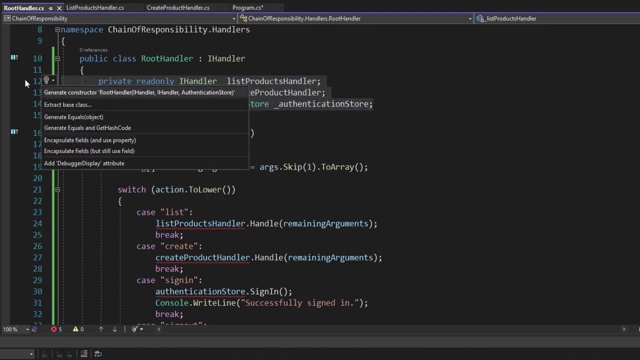 need our list products handler, So let's get that passed in the list products handler, as well as the create product handler. We also need our authentication store passed in So field for the authentication store, So let's get these passed through the constructor and then let's 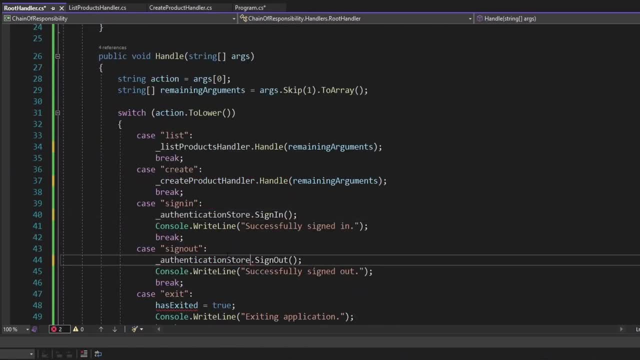 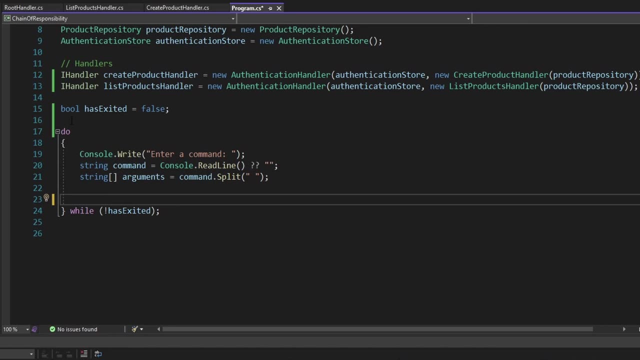 reference them in our switch statement. So here we go. Exit logic is going to be a little bit more complex because we no longer have access to the flag. that's outside of our do while. So for now we'll just comment that out, but we'll come back to implementing. 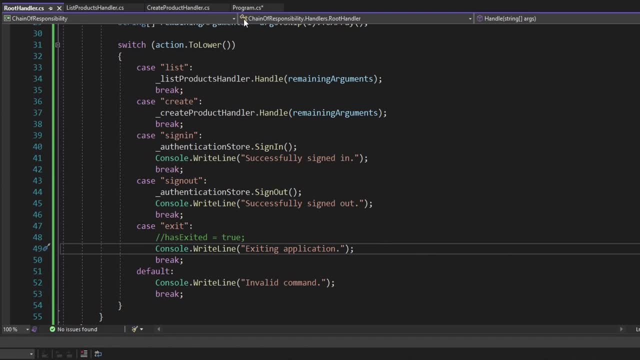 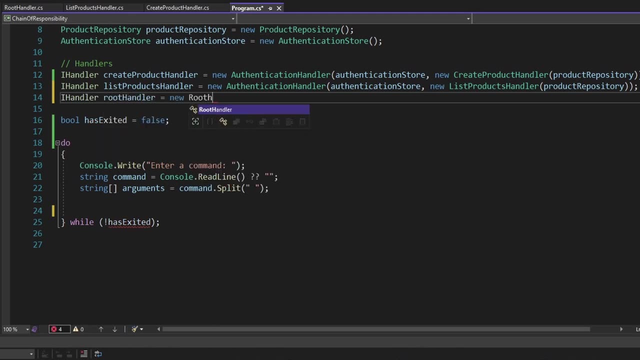 this. I want to make sure we have feature parity in the before and after of introducing this pattern. So now in our programcs let's create our root handler. So just instantiate that. pass in our list products handler. create product handler and the authentication store. So now we're just going to. 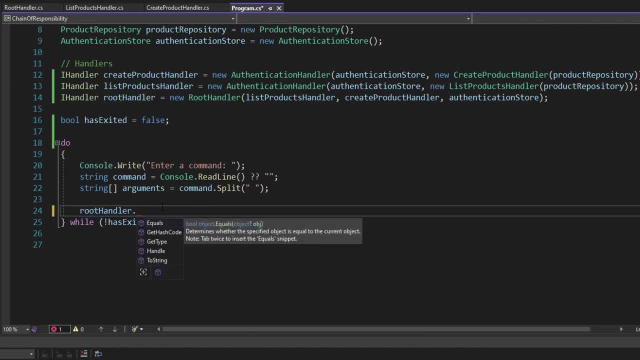 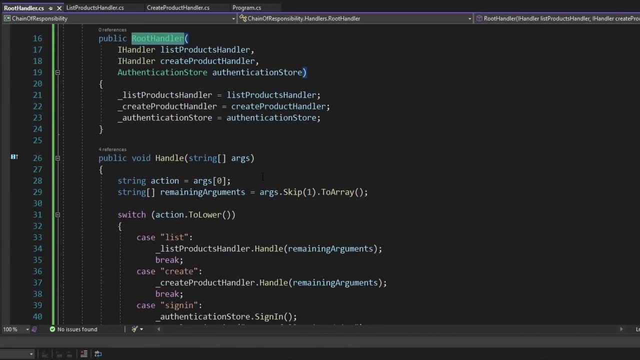 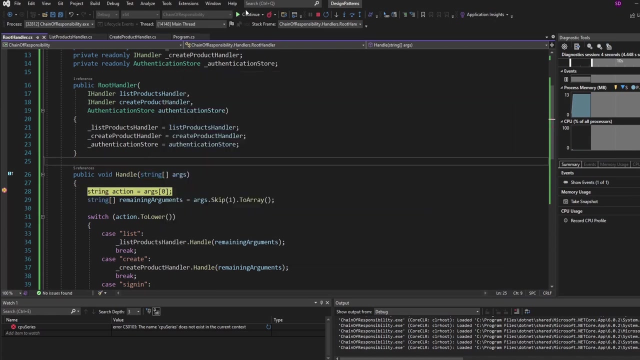 have to use this handler. So let's pass in the arguments that we get from the command that we type in. So let's pass in those arguments and these will get funneled into our root handler. So let's put a breakpoint here and test this out. So let's sign in. There we go, We hit our root handler and this: 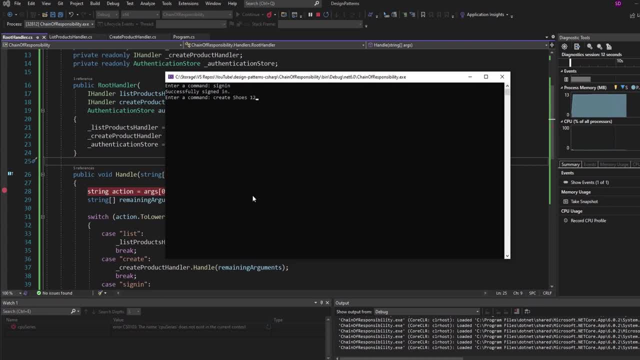 should work just fine. Let's create a product- So shoes 120- and hit our breakpoint. again Let's remove this, and this works just fine. Again, let's list products: There we go And let's exit, And that doesn't work. but we'll come back to that. So now that we have this root, 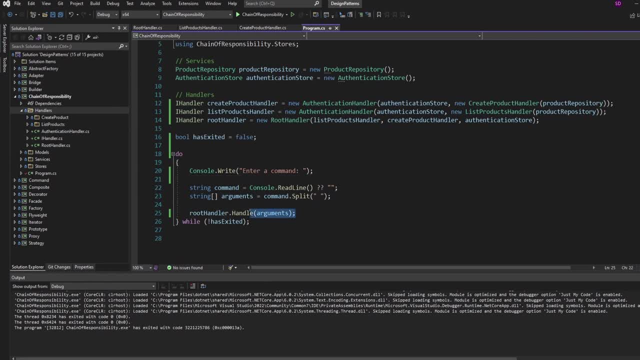 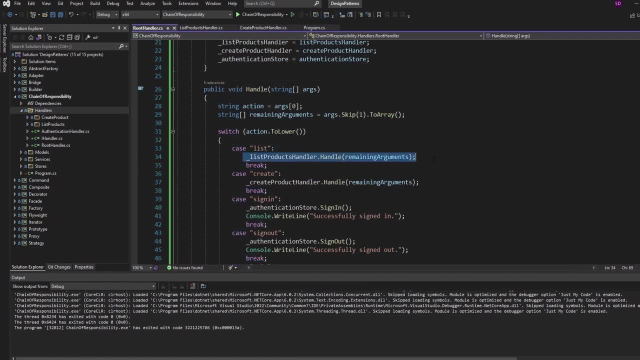 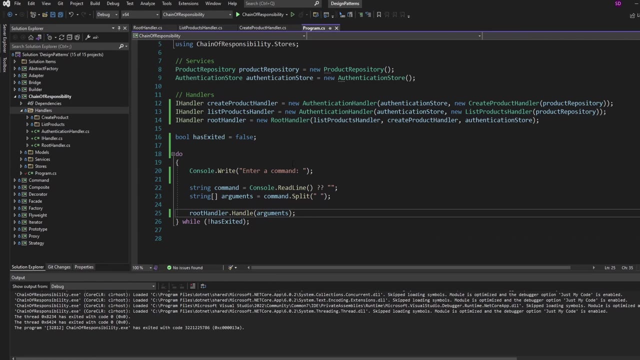 handler. now all the client has to do is pass in the initial arguments, So the client no longer has to handle the complexity of mapping the action name to the correct handler. In fact, on that note, we can implement this exit handler without having to change our client code. So let's do that. 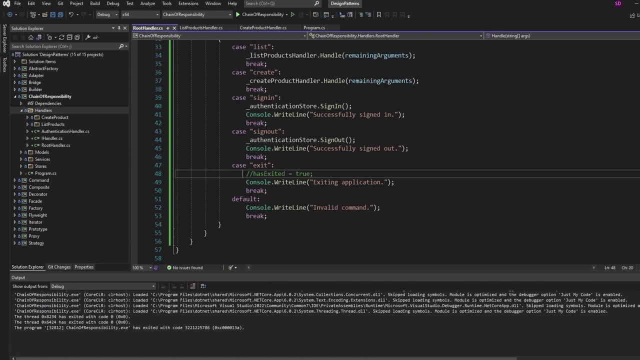 So the way we're handling the exit before is we would set this has exited flag to true, But we can't do that anymore because has exited is outside the scope of this function, of course. So instead we're going to move this has exited flag into an object and we'll be able to pass. 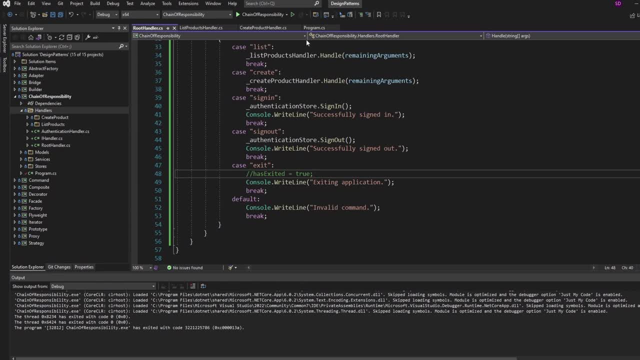 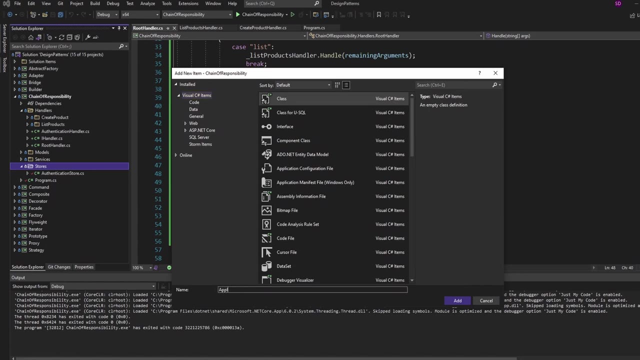 that object around by reference, so that we can access it in our programcs where we need to read it, and in our root handler or any other handler that needs to set it to true. So let's create that, We'll make that a store and we'll just call it the application store. 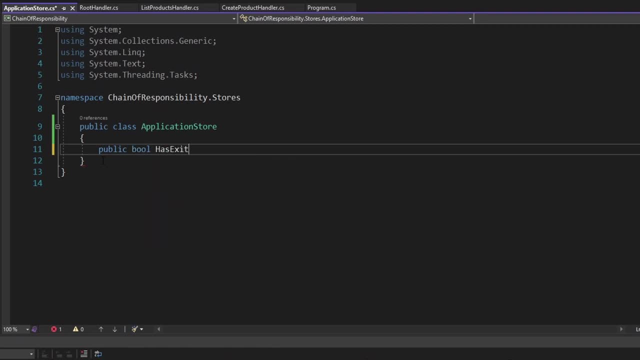 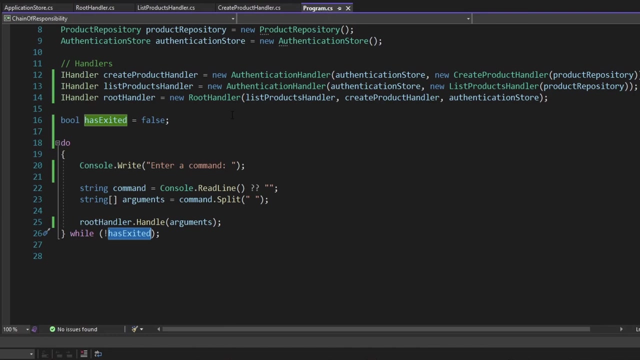 So on the store, we'll have a read only property for has exited, So we'll be able to read it, but we'll only be able to set it from inside the class And then we'll have an exit method where we'll set has exited to true. So let's initialize the store in our programcs. 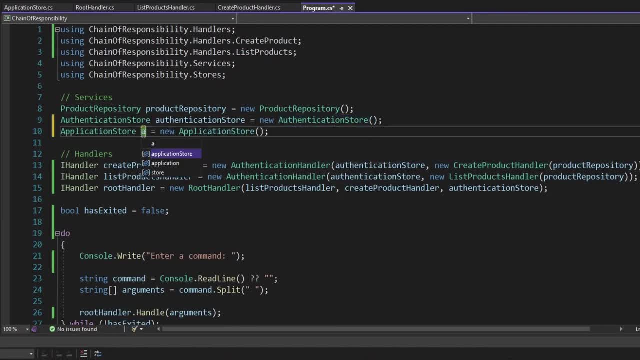 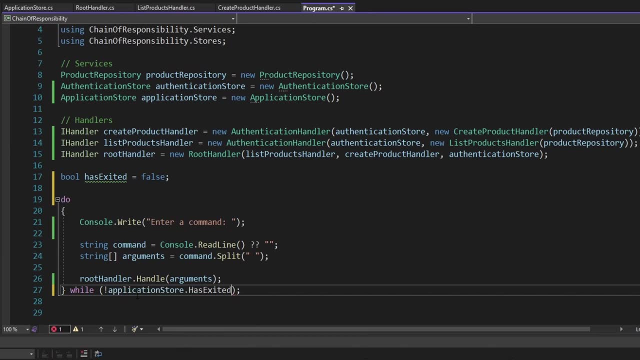 This is the application store, So we'll just name it that, And we only want to continue again through this do while loop. if the application stores has exited flag is false, So I'll go there Now. we just need to set this flag to true by calling exit. 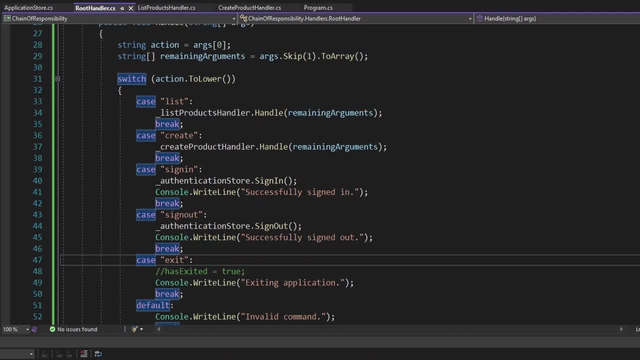 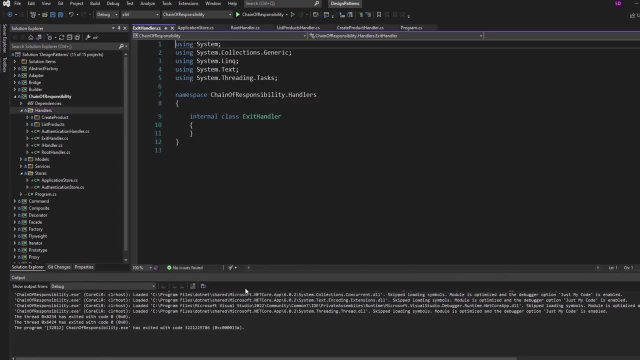 So we could just do that here. but I think I want to continue to make this handler based. So we're going to create another handler. We'll call this the exit handler, and this should be pretty straightforward to create. So we'll implement the I handler interface and then 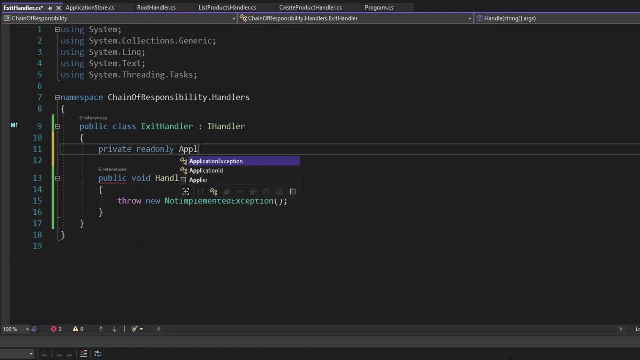 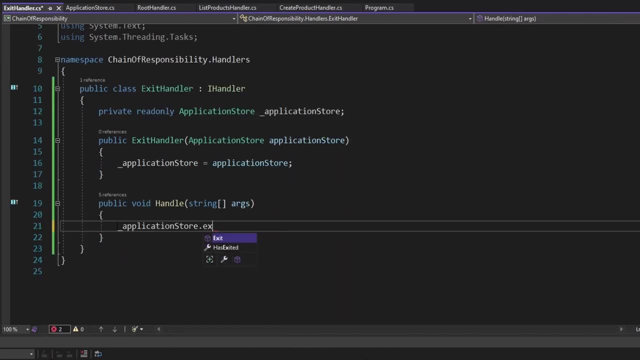 we're going to need our application store passed in so we can toggle that exit flag. So let's get that passed through the constructor And then in our handler we're going to need to create a handler. We'll simply call exit on our application store And we should also write out a console log. 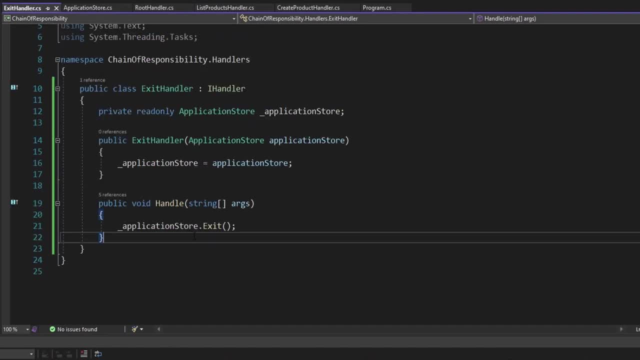 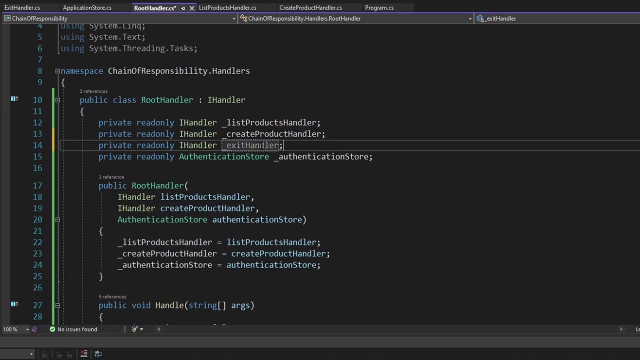 as well. So we'll grab this one exiting application. So pretty straightforward, with this exit handler simply exiting through our application store, which will toggle that flag. So let's use that now. So we're going to get another handler in here. This will be the exit handler. Let's get. 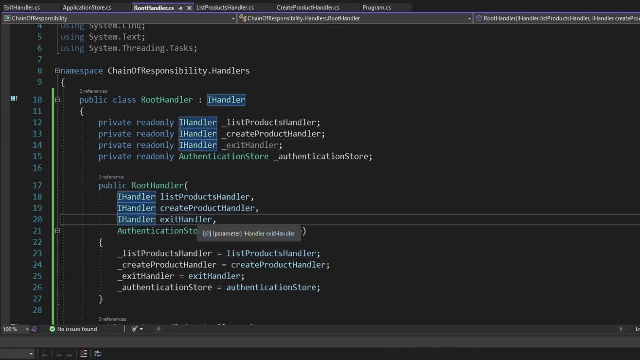 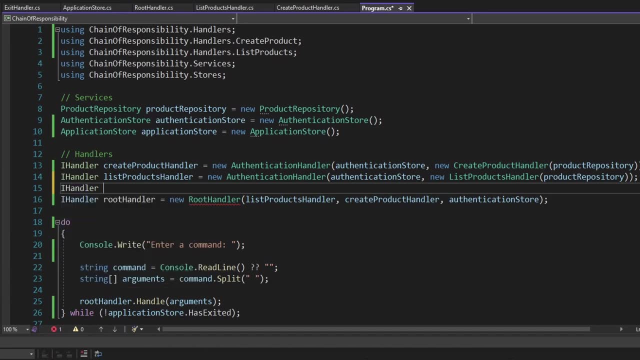 that passed through the constructor. There we go. So now we just need to pass it in when we instantiate this root handler. So first off, let's create the exit handler, So instantiate that and pass in our application store and then just pass in the exit handler to the root handler. 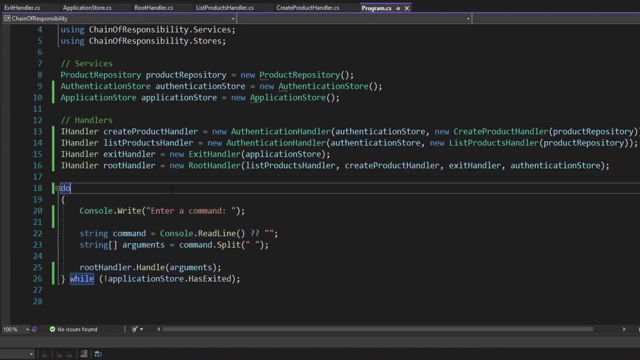 So there we go. We made that change and we didn't have to change our client code. Well, I guess we did, since we're now using this has exited flag on the application store. but that was really just an infrastructure change. In reality, the core logic didn't have to change at all, And I was